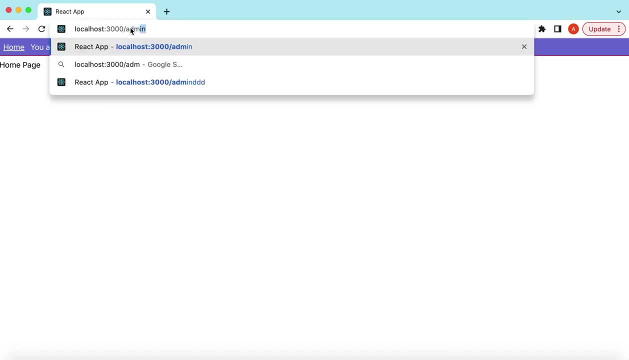 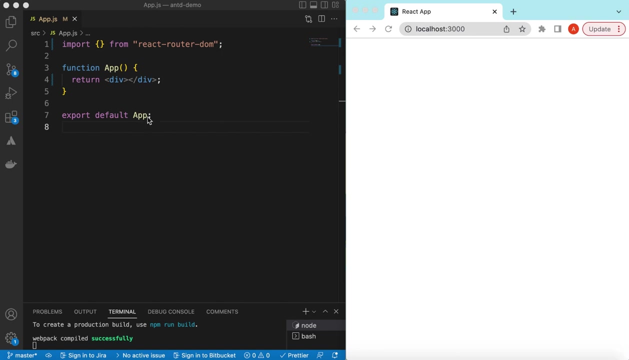 browser address bar. it will redirect me to the home page and maybe if i go to the admin it will say: you do not access to that page and if i type something, maybe abc, it says that this page not found to see how we will implement this role based routing. let's get started. i have an empty reactjs. 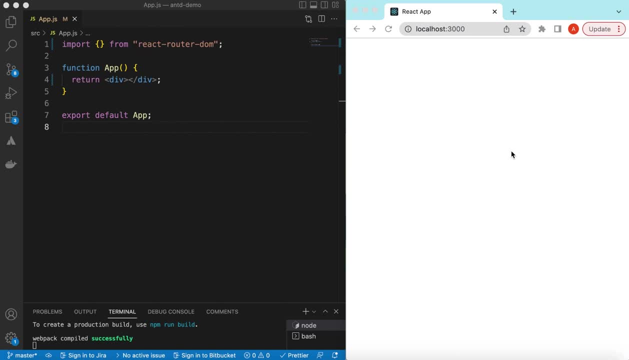 project that is using react autodone and right now it's showing nothing. so let's go ahead and start adding role based routing. so for that, first you need to install the react autodone. you can install that using npm: install react autodone. so once that is installed first, 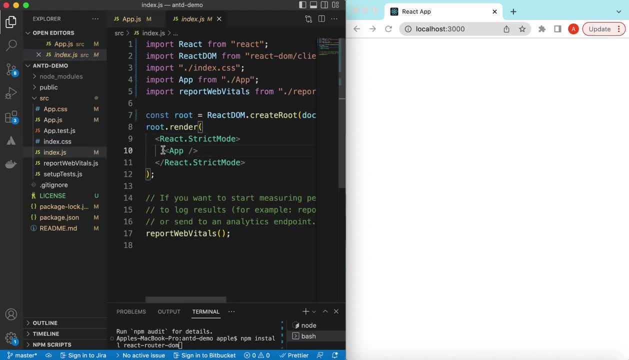 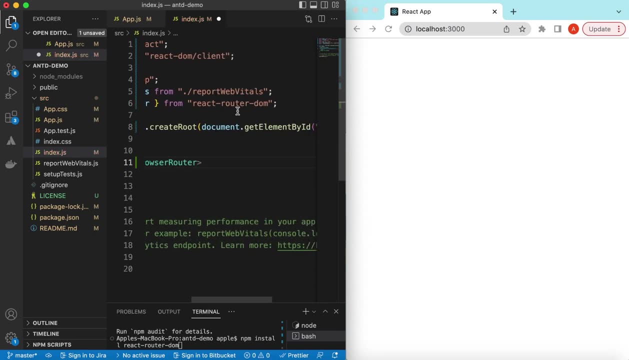 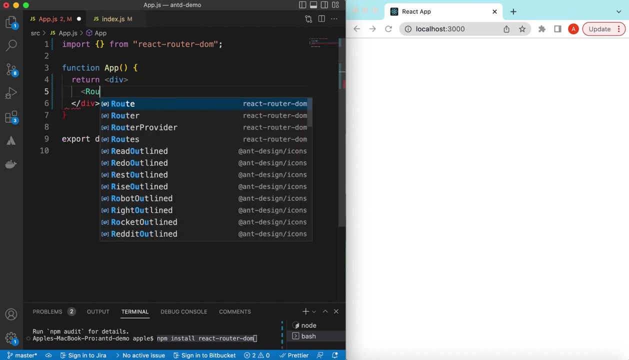 thing we need to do is we need to encapsulate our main root component, that is, the app, inside a browser router. so we can do that browser router that is from the react autodone and cut it from here and paste here. okay, once that is done, we can start using the roads in our app component. so let's. 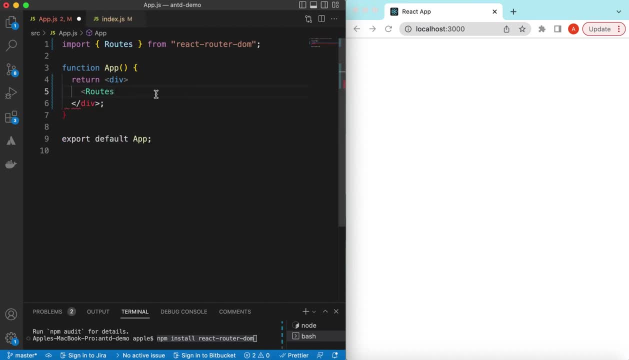 define the roads again, from the reactor to dome and inside the roads we can define a single road and here we can say: for a path, if it is a single slash, or we can say the home, what element we need to render. so suppose in that case we want to render a home component. 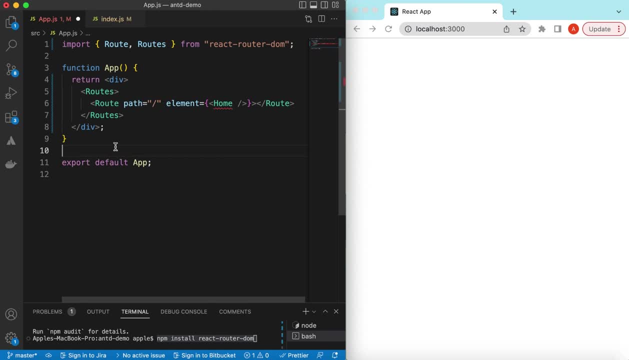 and let's define this home component as well, so we can say: function home and we can return maybe a simple div. we can say home, if i save it, here you go, i'm on the route and this home is shown. right, let's add a few more roads. uh, we can say, if it is like, 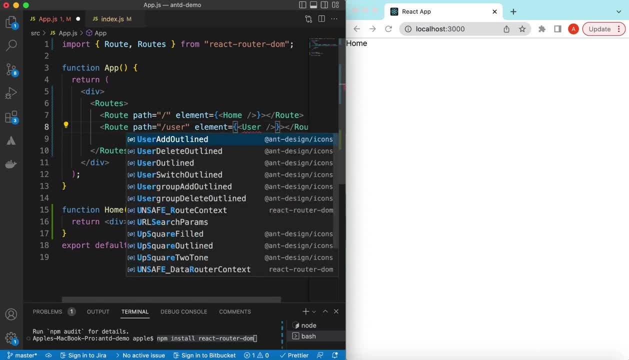 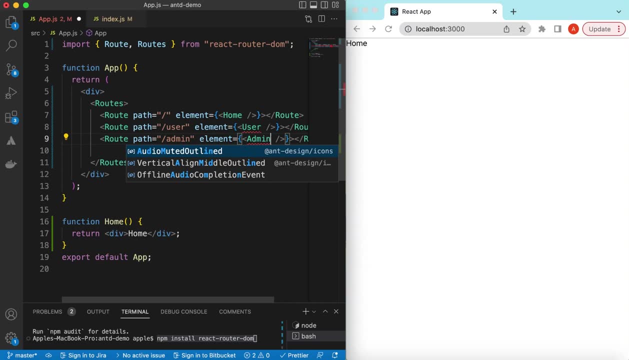 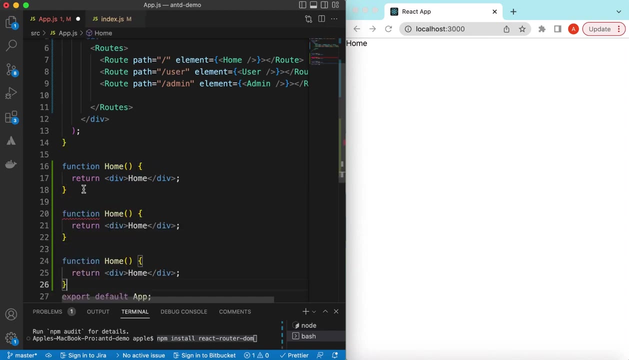 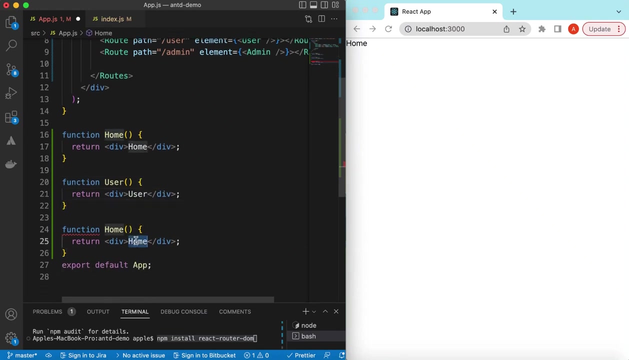 under a user, we want to show a user component, and if it is, uh, admin, we want to show a admin component. right, so let's copy this one and add those components as well. we can say user and here we can say admin page, maybe admin, and you can say: this is a user page, maybe you can. 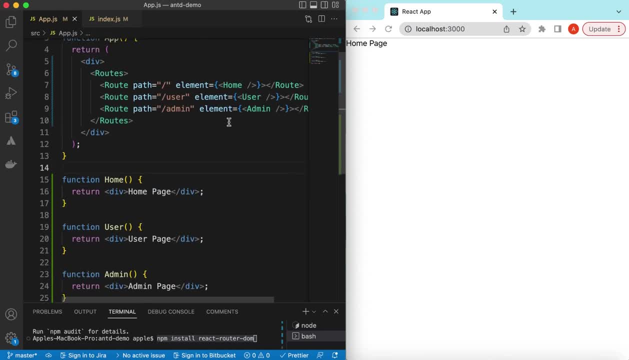 say home page: right, save it right. if it is a home page. and if i go to the user, it's a user page. and if i go to the admin, it says admin page- right. and if i go something which is not there, uh, it shows empty. we can write something here as well. 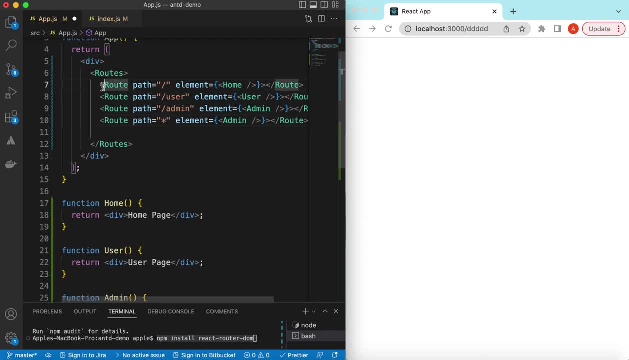 so we can say in case of the roads, if it is not between these routes, slash as slash, user as slash admin. if it is other than this, we can say inside a div: maybe you can say: page not found, right, save it, go. it says page not found. so right now, you see, i can access any of these routes. so if you want to, 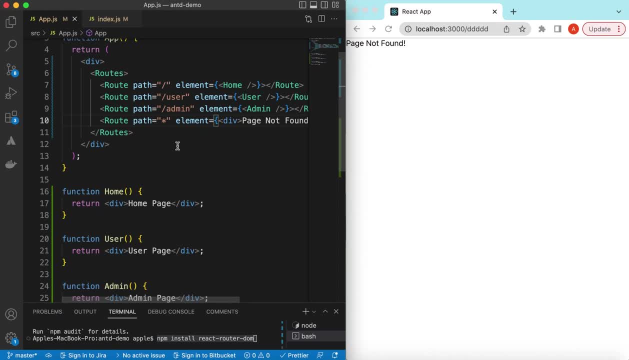 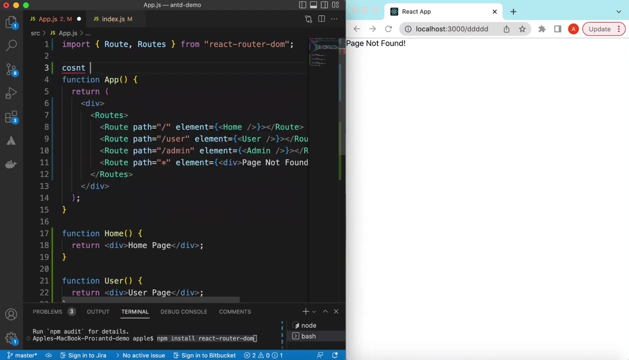 make them role based. like if i am logged in as a normal user, i should be able to access only this user or the home, and if if i am an admin, then i can assess all of these right. so for that we can mimic the behavior and we can create a constant here. we can say cost, cost. 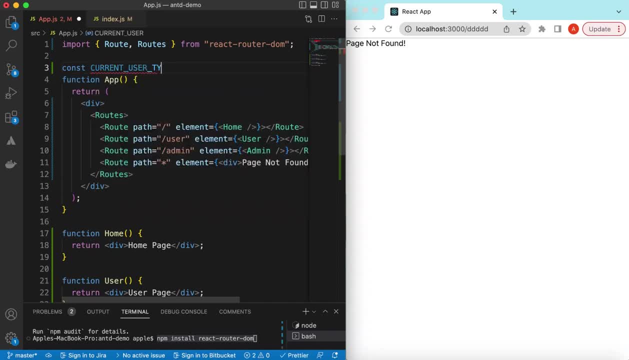 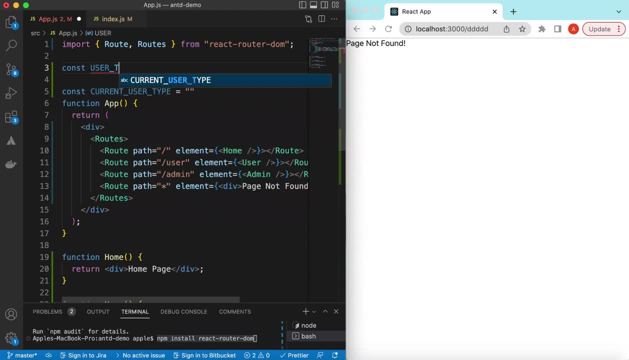 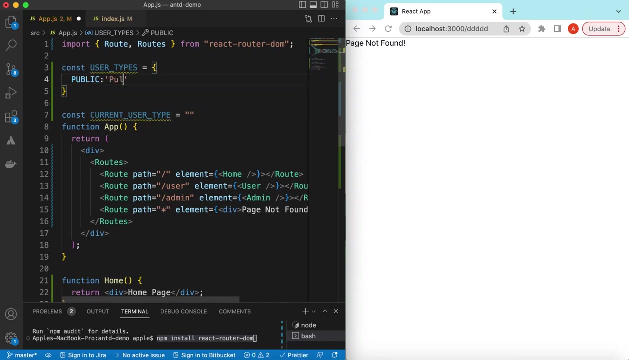 you can say current user type and we can define some user types as well. we can say const user types and here we can say it is a public user, and maybe then we can say, uh, normal user. right, a public user will be only able to access this home and the normal user will be only able. 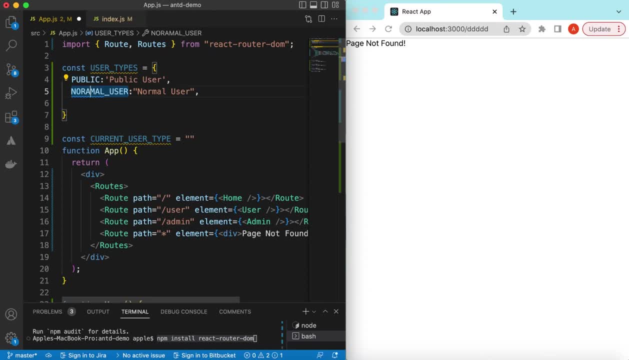 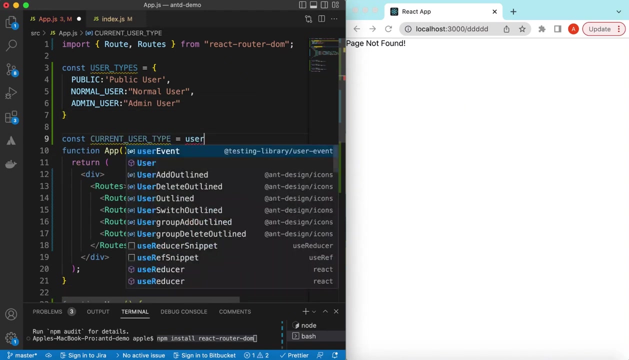 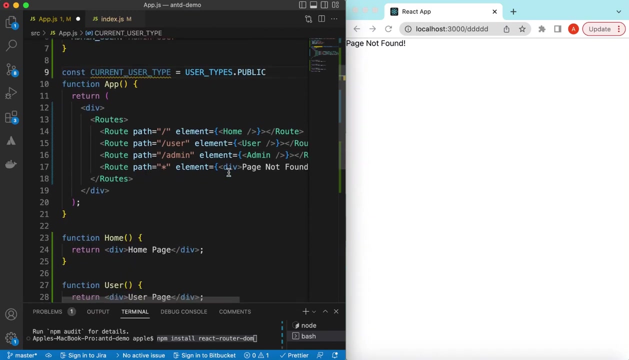 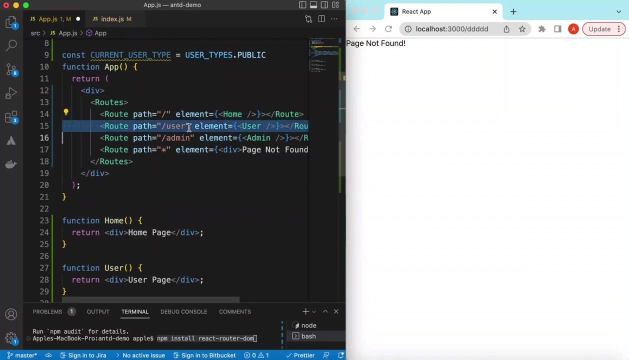 to access this user as well as this home, and then we can say: the admin user and this user should be able to access all of these pages, right? so by default maybe we can say user types and we can say garbage, isoster, its single admin user, and here we can say we can define, uh, some elements. we can say this is a public. 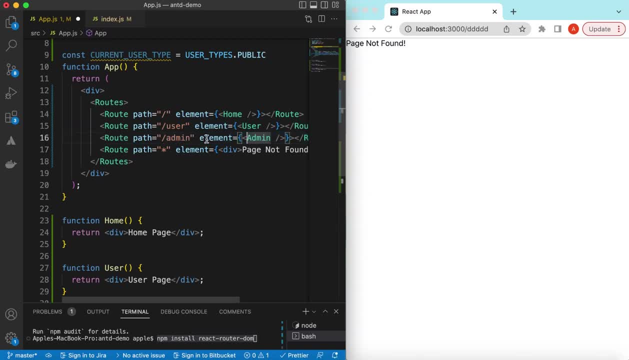 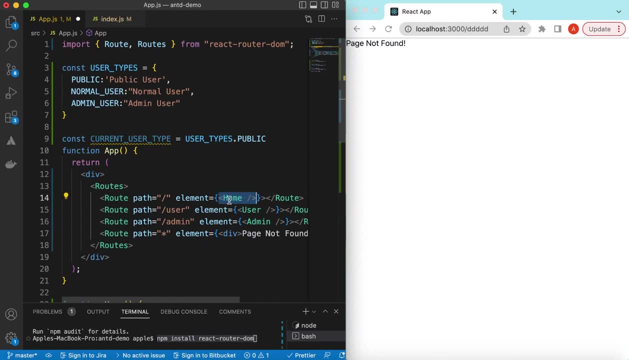 element. this is a normal user element and this is, uh, you can say, the admin element, right? so while returning this, these elements home, we can encapsulate them inside some elements. we can say this is a, we can say, public user element. that's right. see the page and the keyword need to be. heric. so i can say we can say foods and indeed content, right, so this is our whichever type of item. let's say I need to insert that new item, so tree fit field and I will insert some items at this screen here. lets say book, type it now and with this above I can insert. will beрокie. I mean its like a within the title. see, I will have an alpha. is that it is something that's great and bars of refers to those. I recommend a change, or it's subject, and it will proceed to a 아니야 in my video. 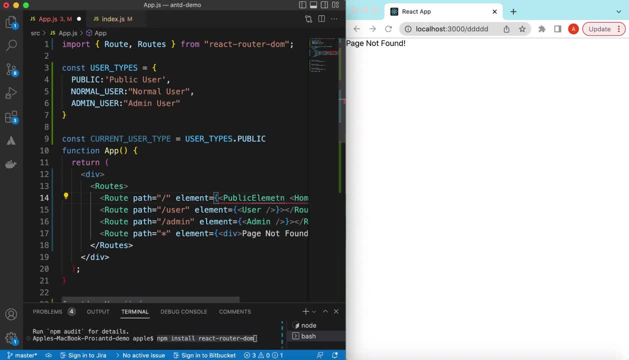 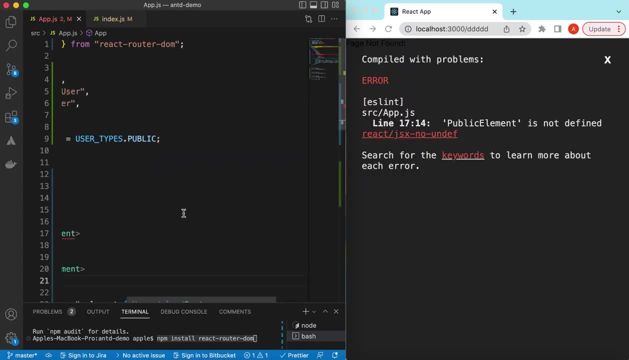 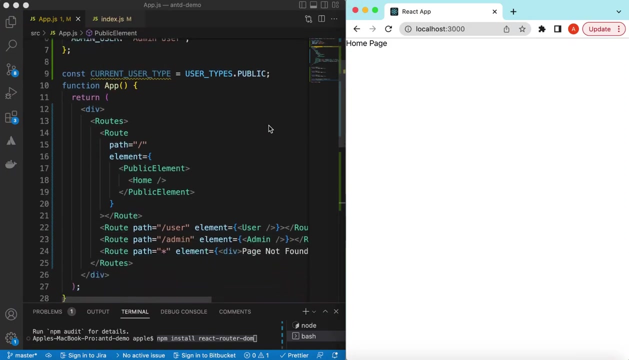 public element. right, if i cut it from here and paste it here, right, and we can define this public element here. here we can say a function and public element and we will be getting the children here and we can return just the children, right, save it. and if i say to home, this is home page, right. 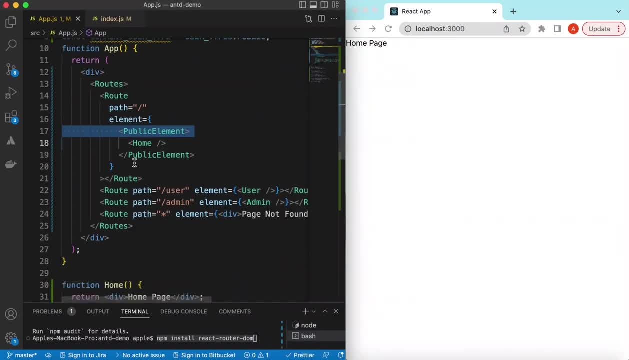 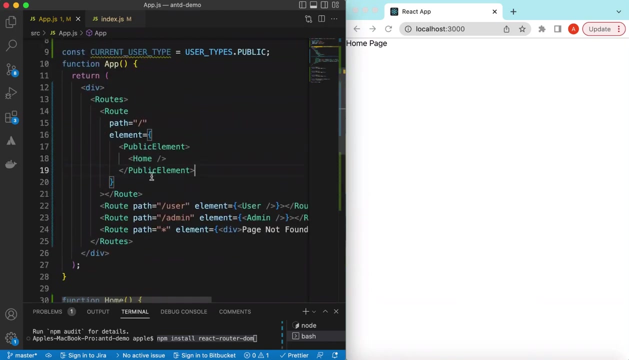 so we have defined, defined a public element. so for all of the routes that you need to be accessible for any type of user, you can encapsulate that inside a public element. or even you can skip this public element as well, because we are just returning the children. whatever is inside that. 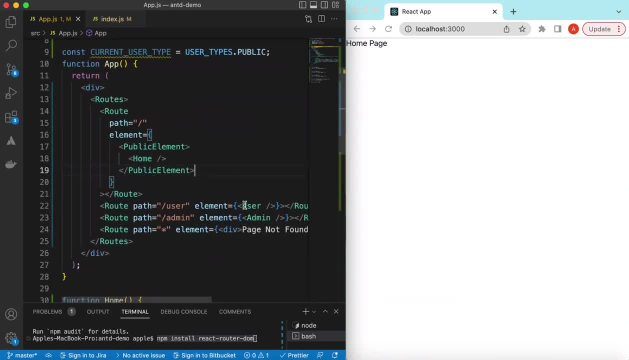 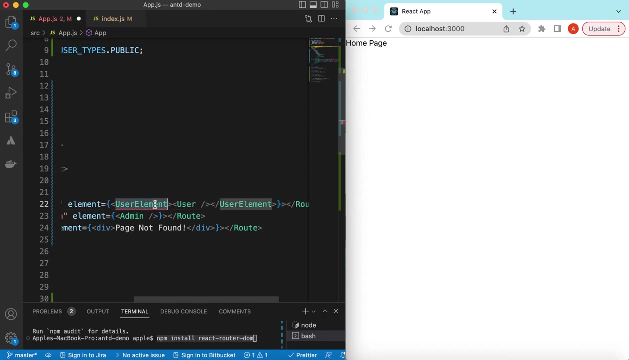 but. but to make it a symmetry, uh, we will be adding the elements. here we can say user elements, then the element elements, right, so we can copy this one, and here we can say public element instead of the public. we can say user element, right, and we can define this user element here. 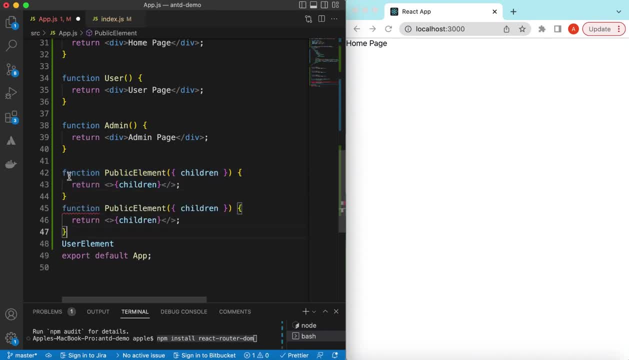 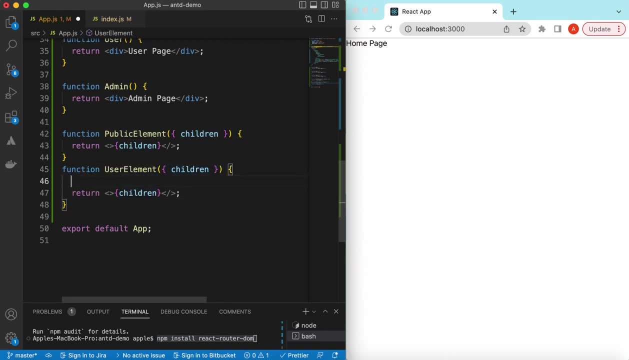 maybe we can copy this one and cut it from here right and here instead of the this children. we will be first checking if the current user type is something we can say- user types, dot. admin user or it is a normal user- then we can. it is an admin or the normal user? 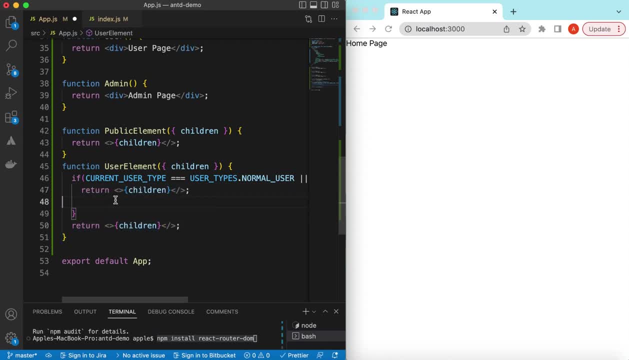 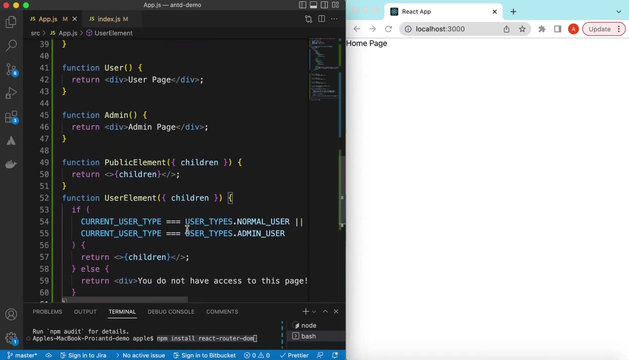 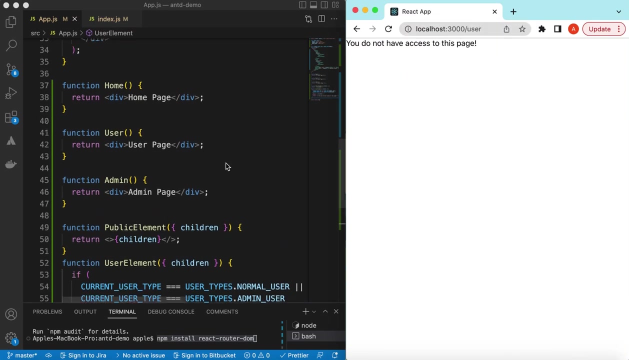 then we will be returning the children right. otherwise we can uh return anything else. maybe we can say: return uh, div. we can say you do not have access to this page, right? if i save it. and now if i go to the user, it says you do not have access to this page, right. 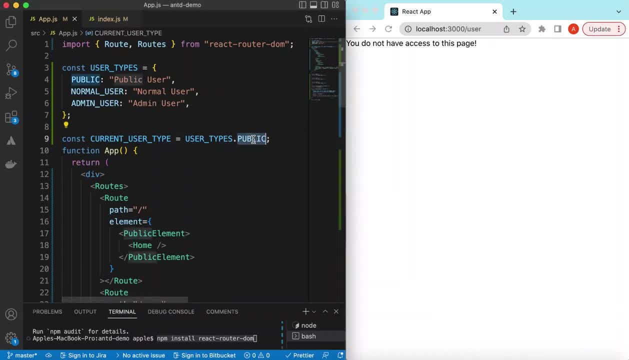 because i am logged in as a public user and if i change this to a normal user, if i save it, it says that, uh, the user page has been rendered right. so that means you have access to this page, right. and if i logged in as an admin user, still, i will be able to have access to this user page. 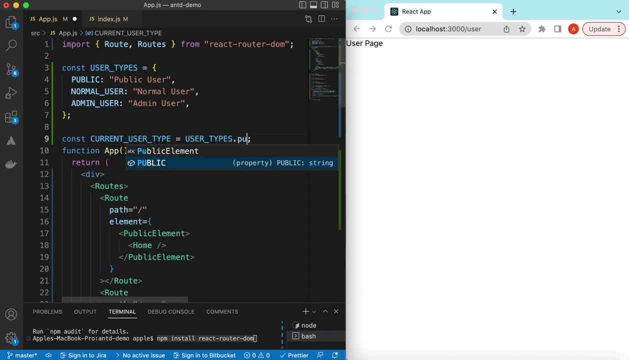 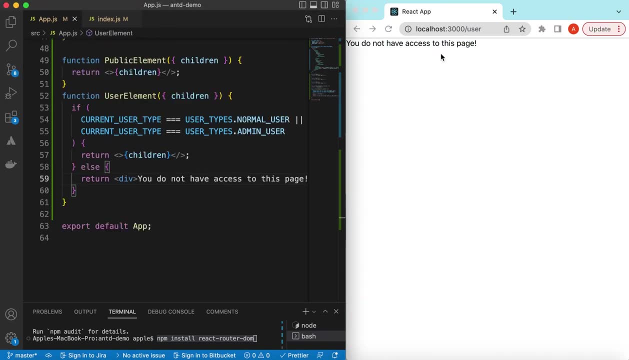 right, and if i again back to the public, so it will say that you do not have access to this page, right? and in in this case, if user does not have access to a particular page, we can show, uh, simple tags or we can navigate to our different page. maybe we can navigate user back to the home. we 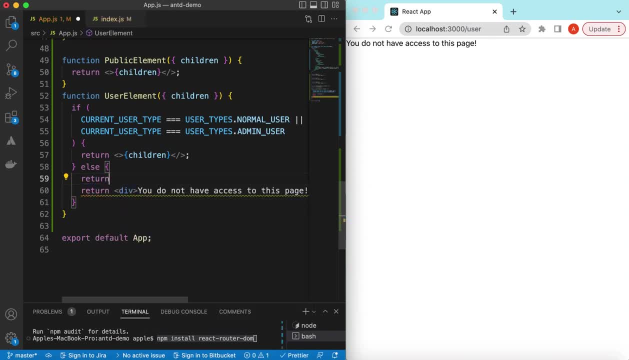 can do this, that as well. we can say return, uh, navigate, that is again from the react autodom. and here we will be providing the two. we have to navigate. and we can say: navigate to the this home, and this will not be executed. okay, here you go. so if i now go to the user, it will navigate me to the 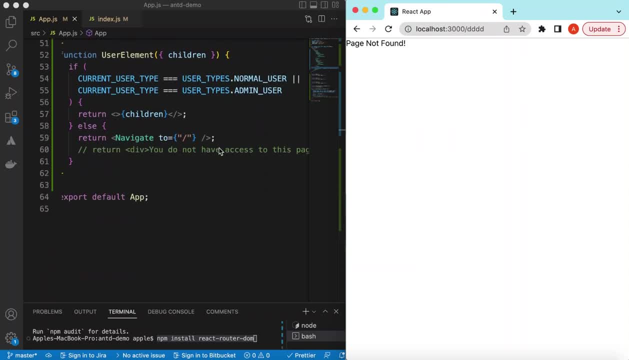 home page. so we can either uh, keep the user on the same page and we can show the message, or we can navigate the user to some other pages. right, or maybe. we can navigate the user to maybe. we can say page not found right, save it. and if i go to the maybe user it says page not found right. 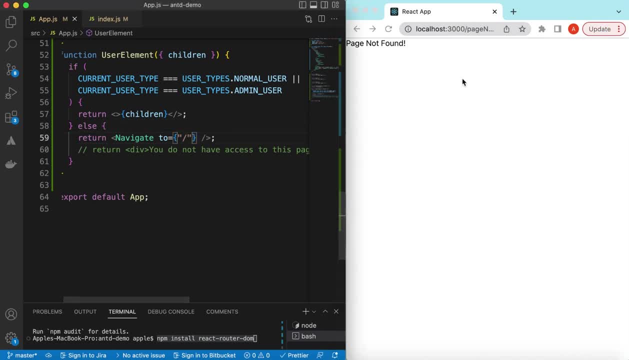 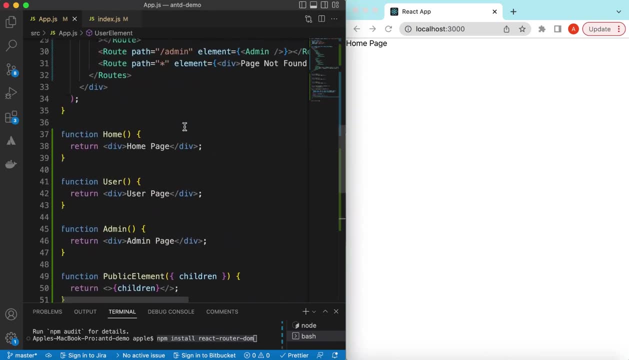 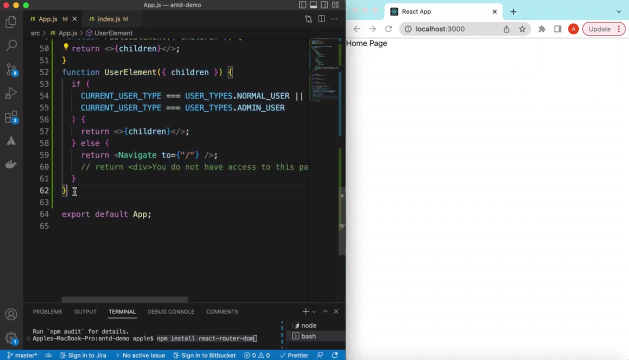 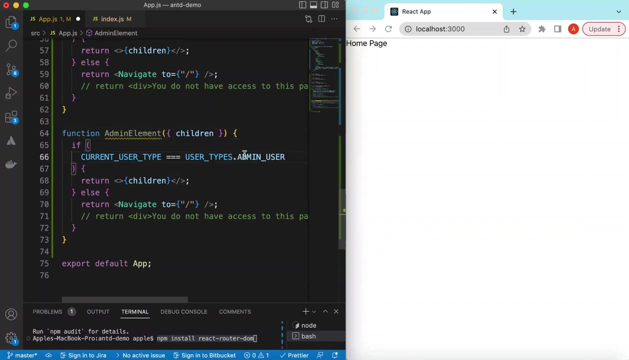 instead of the home right, and if i make this to home it will say home page right, okay, so similarly we can add a element for the admin as well. so maybe we can copy this user element and here we can say the admin element, and it will have only access if it is the user type is admin user, and then we will be showing the children. 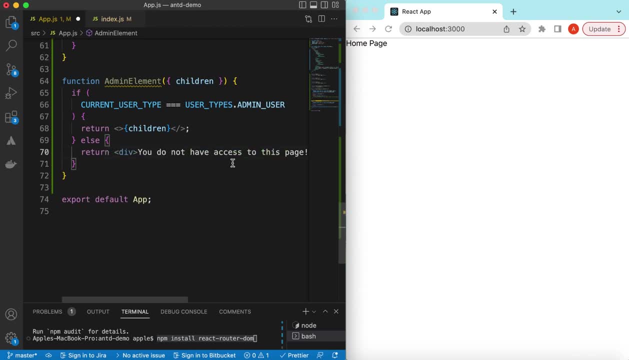 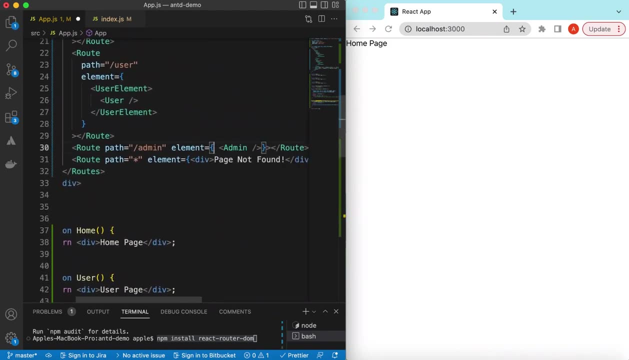 and instead of navigating, we can here we can say: you do not have access to this page, right. and while we are defining our route here, we can say: it is a admin element, right, you can cut it from here and paste it here. okay, so for admin element, we can say admin element. 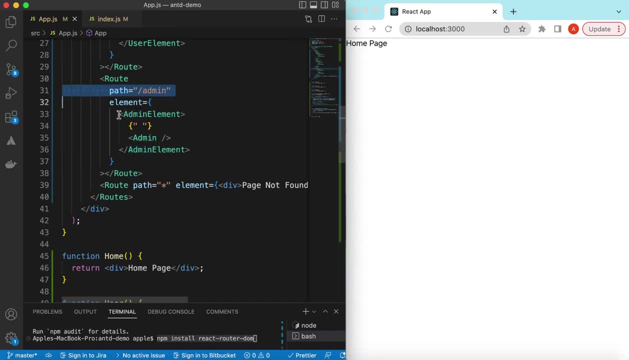 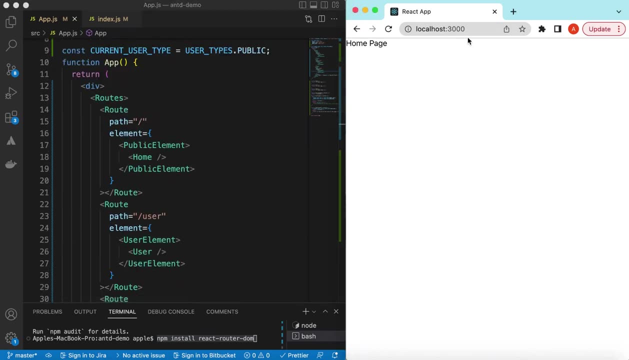 and paste it here. okay, so for admin element: we can cut it from here and paste it here. right, and now we can paste here. okay, so for admin root: we have returned the admin element and inside that, uh, we are running the admin component, right, okay, save it. and now, if i go to, 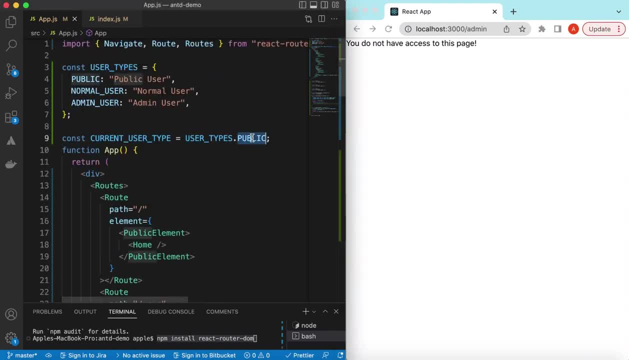 the admin, it says you do not have access to this page. and if i change the user type to the normal user, save it still. it says you do not have access. and if i change this to the admin user, it says now you have access and it has rendered the item p плюс'. but to approve admin. 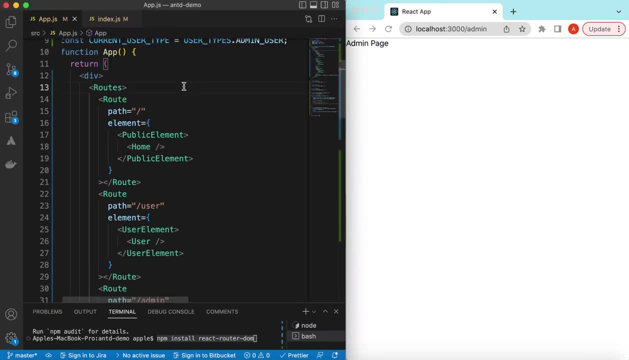 is otherwise. go to custom zeros and go to admin user builder and go to initial yourself and go. so it has rendered the admin page right. so this is all we can create for the admin. Re illustrations can create role-based routes. so we, while we are defining the routes, we 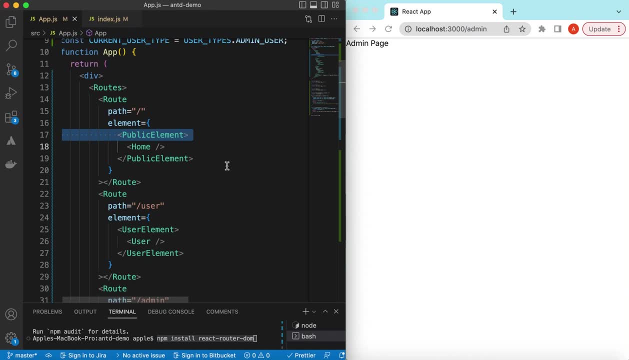 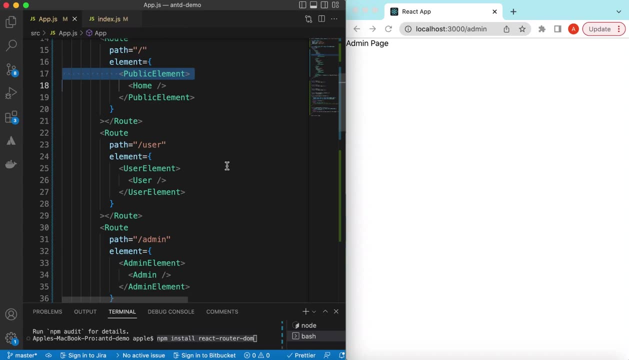 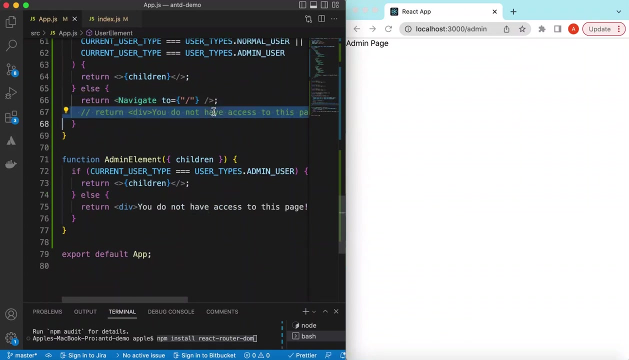 encapsulate those components inside elements and in in those elements we define whether it is accessible for this particular type of user or not. and if it is not accessible, either we can navigate to some other page or we can just show the messages by keeping the user on the on the same page right. so, similarly, if I 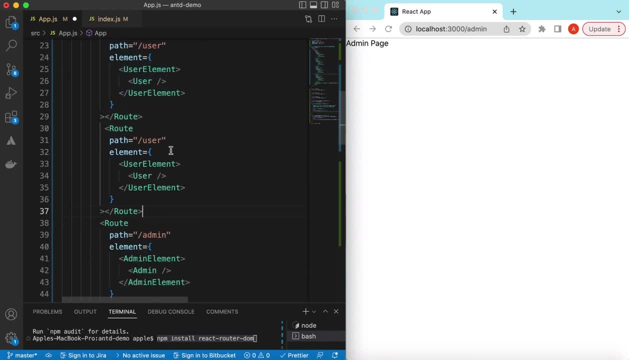 add another route, maybe copy this one, and here I say, instead of this user, I want to say my profile, and it is. you know, if a user element, save it. and if I say my profile, so it should be accessible. right, it's a user page. right, because we just created a new route, but and the element type is the user type. so 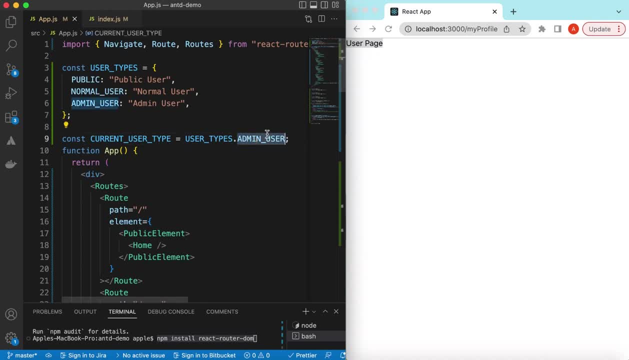 as as long as the user type is admin user or the user type is the user type. so as long as the user type is admin user or the normal user, it should be accessible. but if I change this to public, it should not be accessible. right, it should never get back to the home page because in the 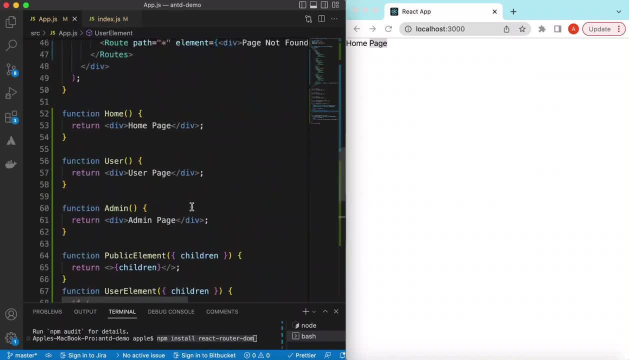 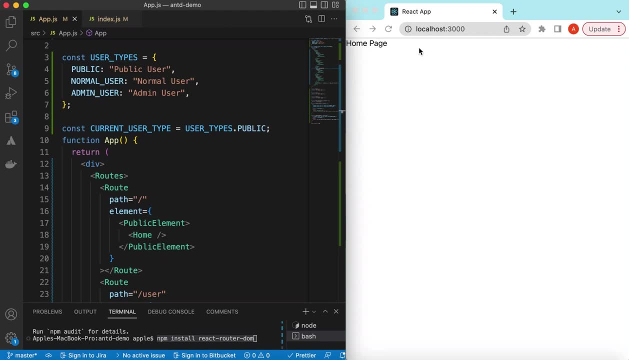 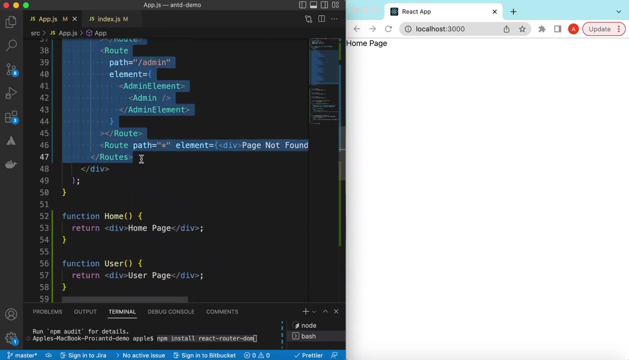 user element, we are navigating to the home page, right? so this is how we create the role-based routing. but if we want to add the links based on the roles, we can add that as well. so maybe for that we can create a simple component for these roles. we can cut it from here and we can create a small function. we can say: 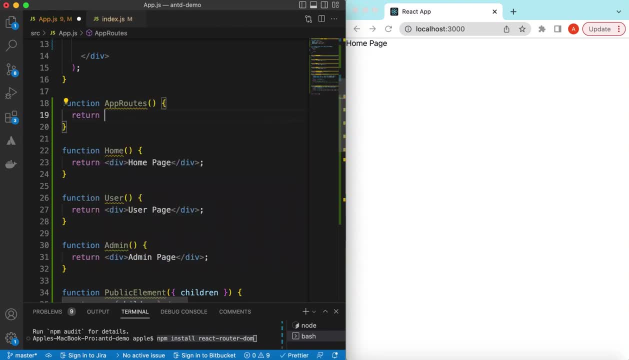 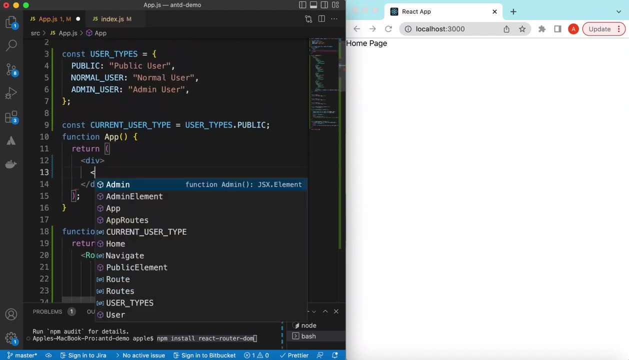 app roads, and here we can return whatever we have written inside the roads right, and here inside the div we can say: app roads, right, it is still the same. and above these rows we can add the links that we can say: maybe inside a div we can say: 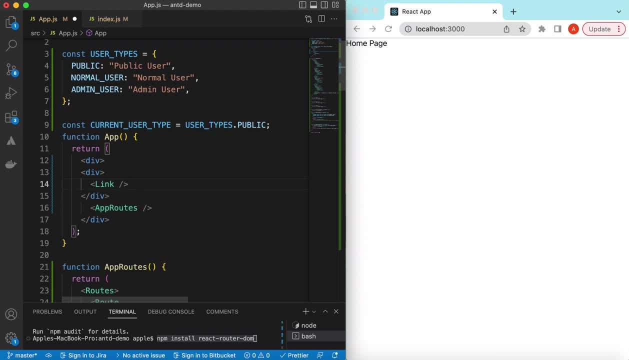 link that will be again from the reactor to dom, and here we can say to go to this home, and we may call this uh home, right, if i save it, there you go. it has added that link and let's copy this one and create the links for other routes as well. so here we can say the user then 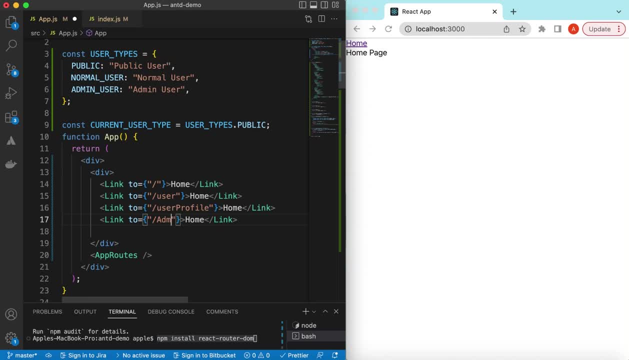 we have the user profile and then we have one for the admin. we can say user and then the user profile and then we can say the admin- right, if i save it and let's add some styling here- and we can say display is flex and we can say gap is. 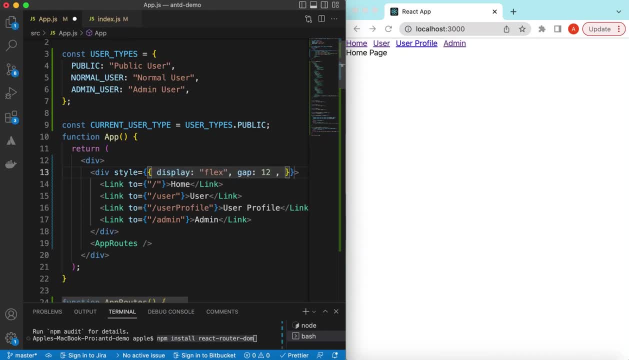 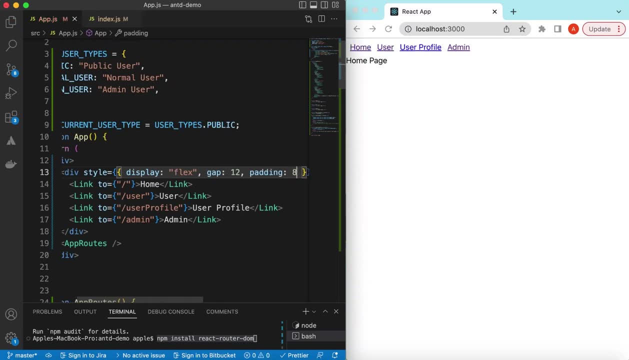 pixels, save it and maybe we can add until padding as well, maybe 24 pixels or maybe only. uh, it is enough. right, and now. if i click off any of these, it will go to that particular page, right, the home page, then the user and, if it changes to admin so that it has access to all of the pages and home. 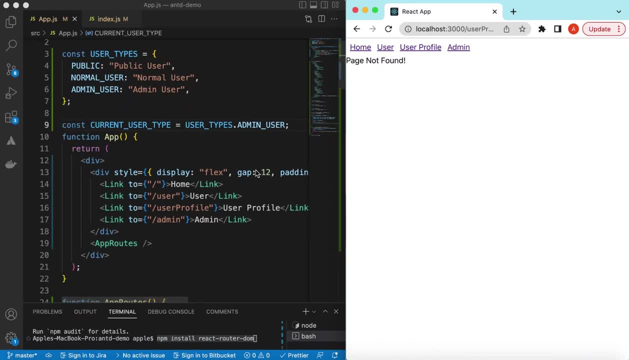 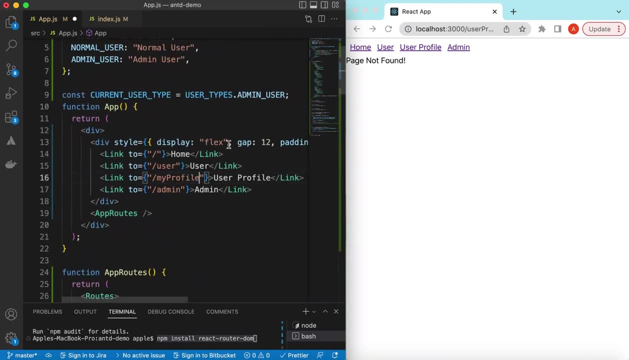 the user page, the user profile. what is inside that? that is my profile, right, save it. okay. use the page and then the admin, right, so it has access to all of these pages. and, uh, you can navigate to any of these right from here and maybe we can uh show your login, right. 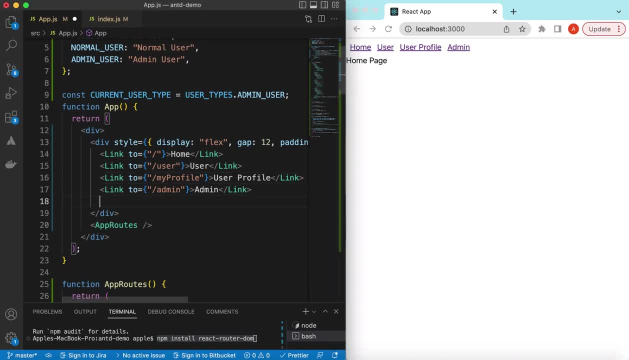 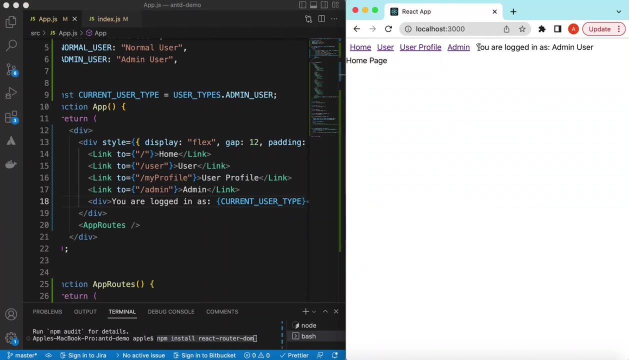 in this way, so for that maybe we can say inside a day. uh, you can say you are loading as, and here we can say current user type. here you go. you are loading as admin user, then you have access to all of these pages. and if i am loading as a public, so for public user i do not have access to the. 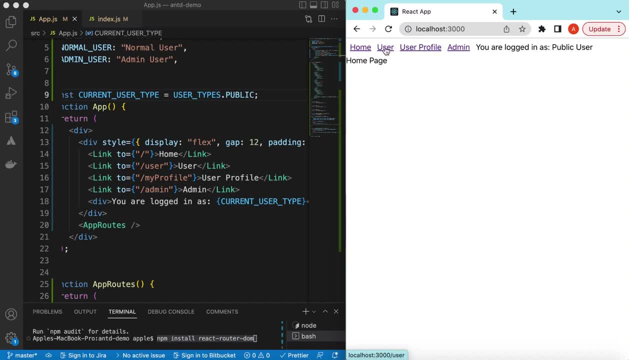 admin, no access to the user profile, no access to the user, and now you only have the access to the, to the home page. i'm. if i click on any of these, it will navigate me to the home page right. and in case of admin, we are saying that you do not have access to this page right. and if i uh, normal. 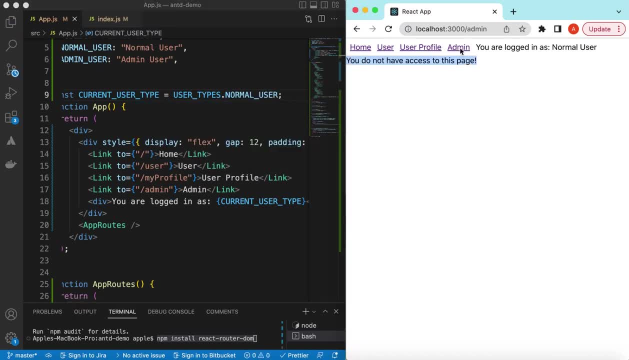 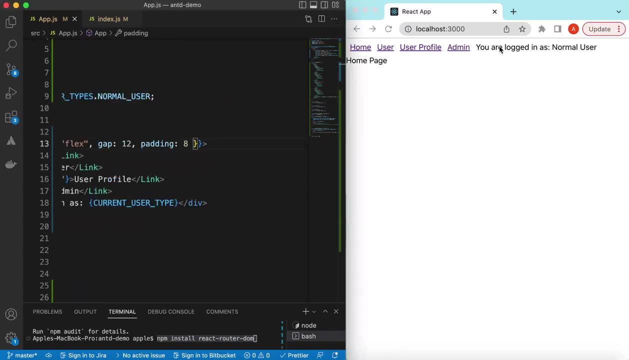 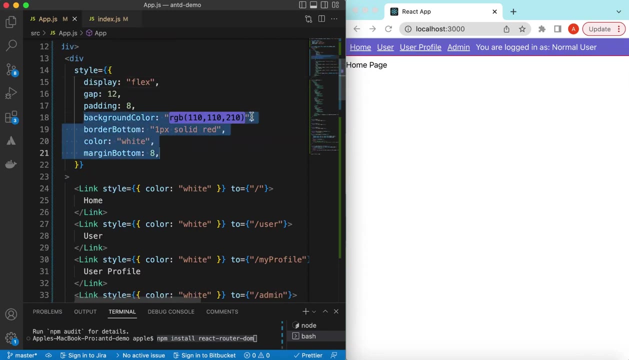 user, then i should not access to admin, but i have access to user file as well as user and the home page. right, let's add a little more styling to the header to look a little better. so i have added a little styling. so i said background color this one and added a bottom border of red and made 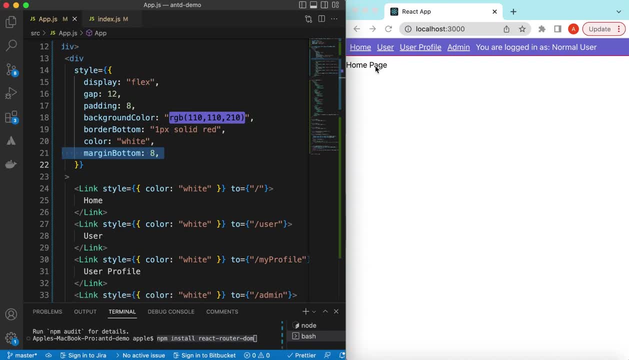 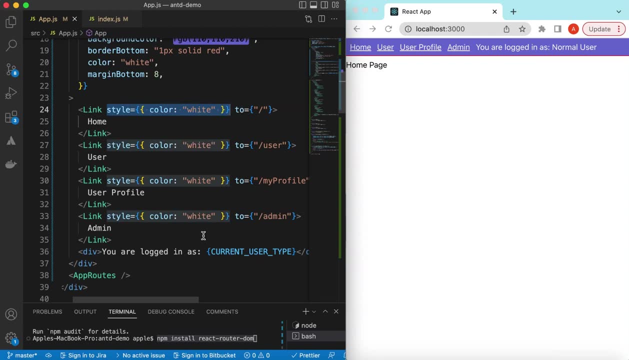 the color to white and add a margin bottom to eight pixels, and then i have also added the style to all of these links and made the color to white right. and here you see, we are always showing, uh, the links in the header and if you want that, we want to hide the links which are not applicable. 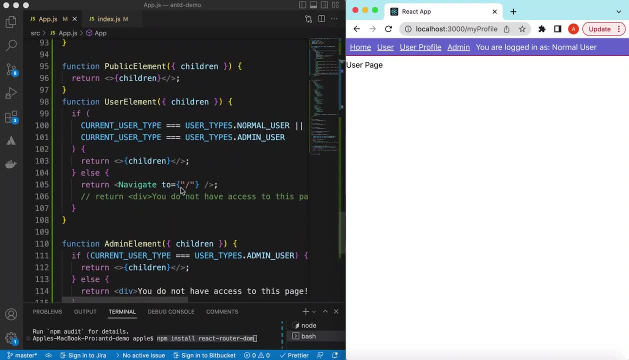 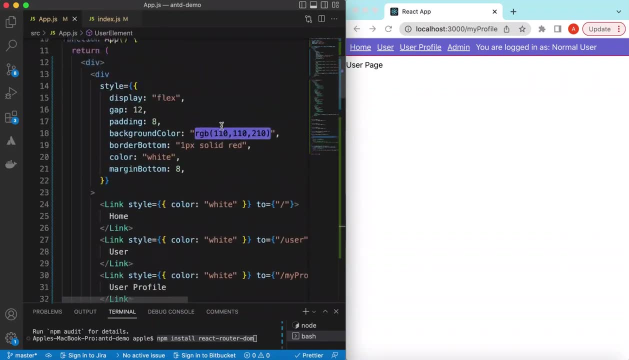 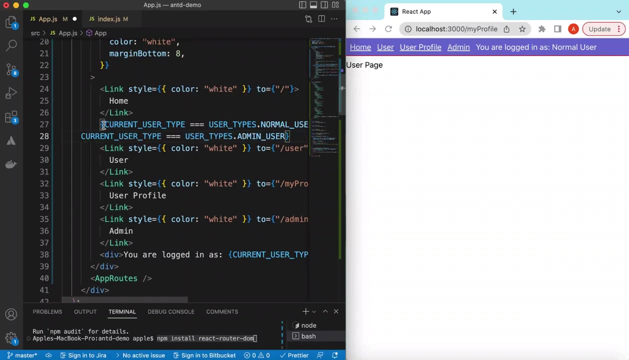 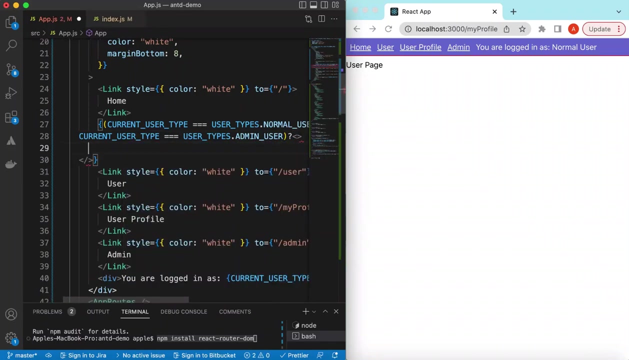 we can do that as well. so we will be doing the similar work we did for the uh, defining the user elements, so we can copy this condition from here and while we are showing these links, so then we can say here: if it is this user type, then you can show that inside a fragment. 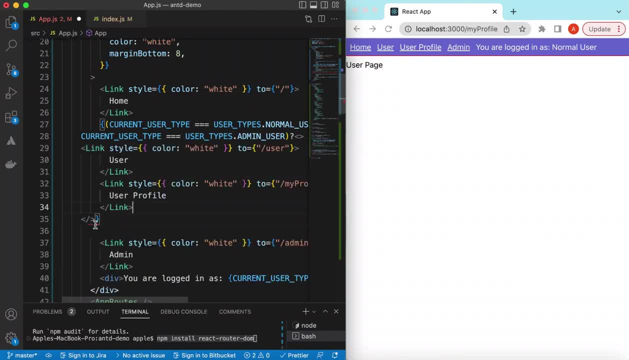 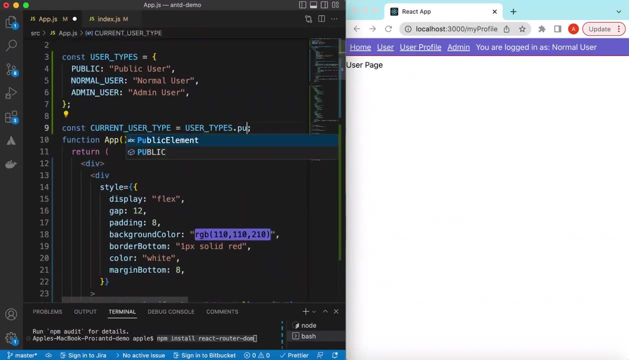 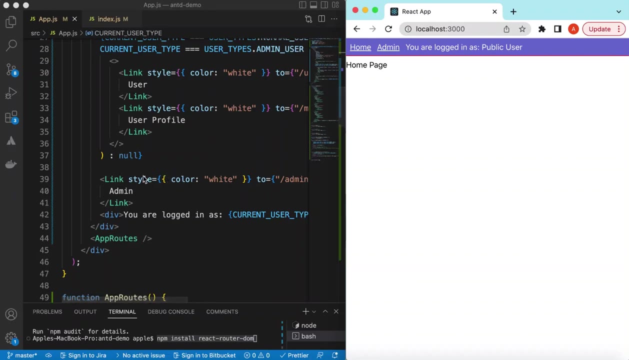 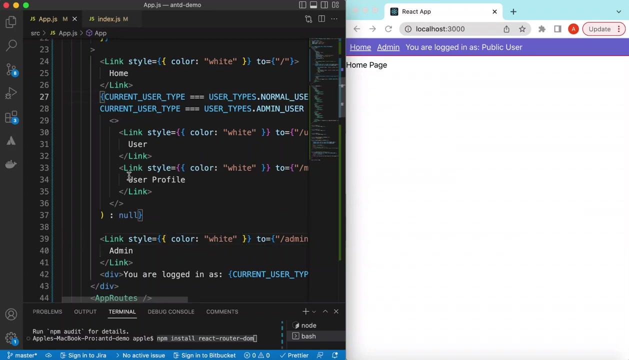 these two links, cut it from here and show it here, and otherwise we can say: show null, right. so right now i am a normal user if i say it's public, so the user and then the user profile is not shown here, right? and similarly we can do that for this admin as well. so let's copy this one and 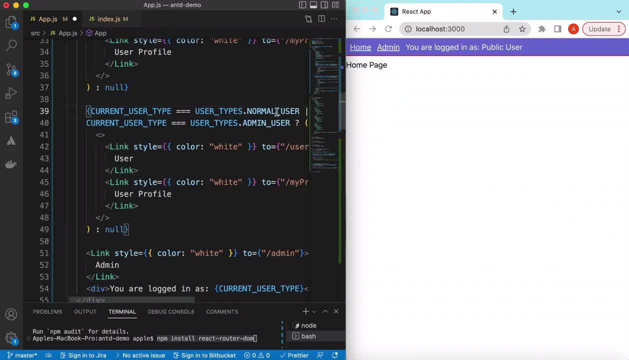 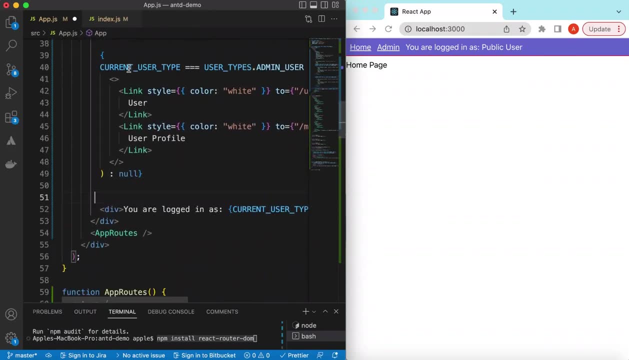 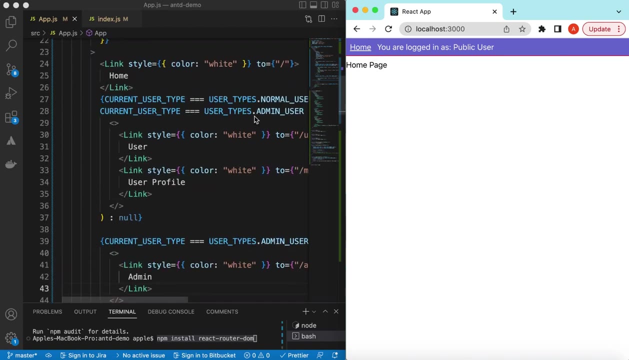 paste it here and here. we can only say: if it is a admin user, then we can show this particular link, right? otherwise don't show so it it has not shown the link and we cannot not even go from here as well. right, it says admin. is you do not have access to that page, right? and if i'm, uh, the admin? 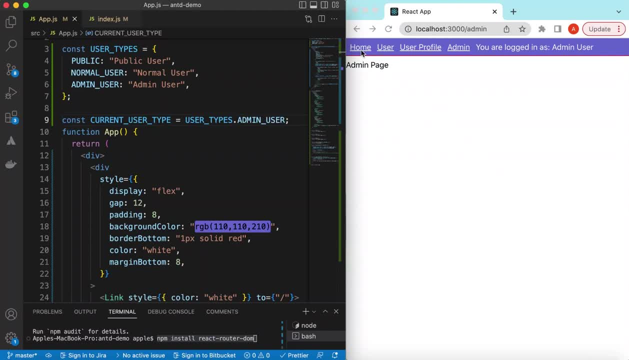 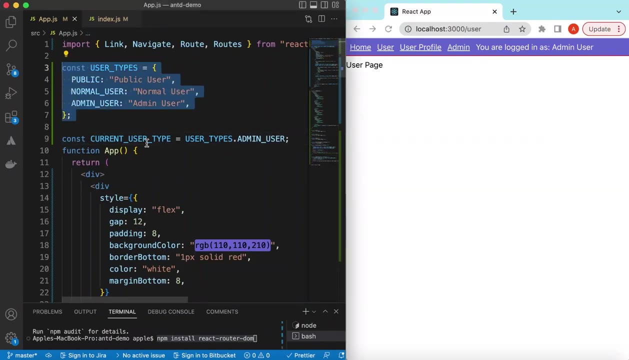 user, save it. it says that you have access to all of these pages, and i'm then, uh, go to any of these from here, as well as, uh, from browser dashboard. so, as a summary, what we did is, uh, we have defined the user types at the very top and then 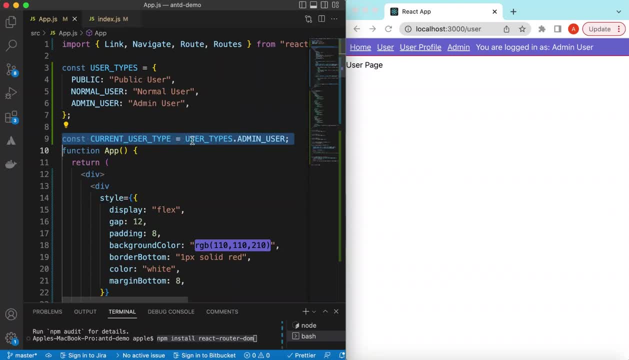 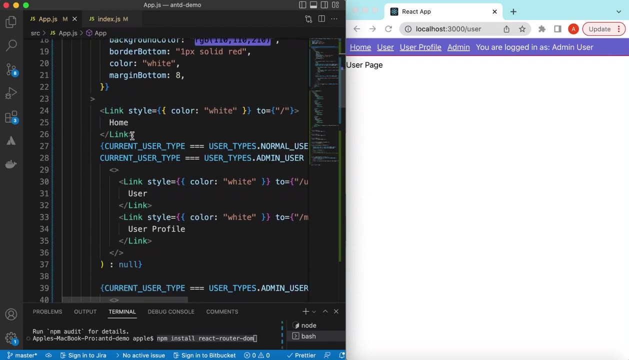 we have defined the current user type. so, uh, we mimic the behavior here by defining our constant, but in actual uh use case, you will be having your uh current user type inside. uh, we can say redux, reducer, or in uh global state or somewhere right, and then uh we 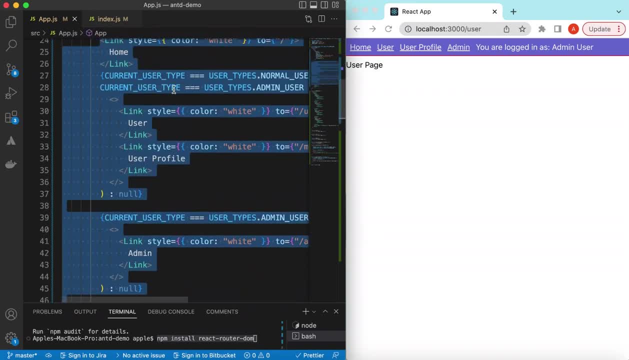 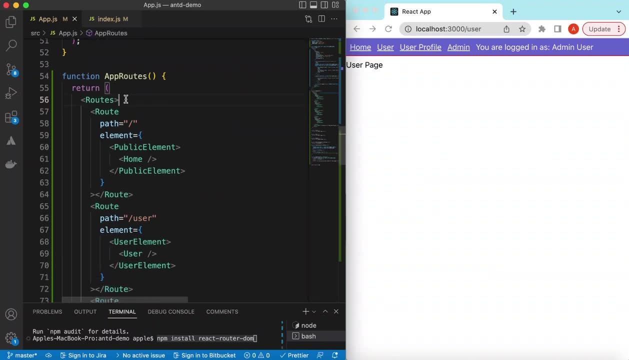 have defined our links- uh, for the header- and there we have added the conditions when to show: show those links based on the current user types. and similarly, we have defined the app routes and while defining each app route, we said: what is the type of that particular route, if it is? 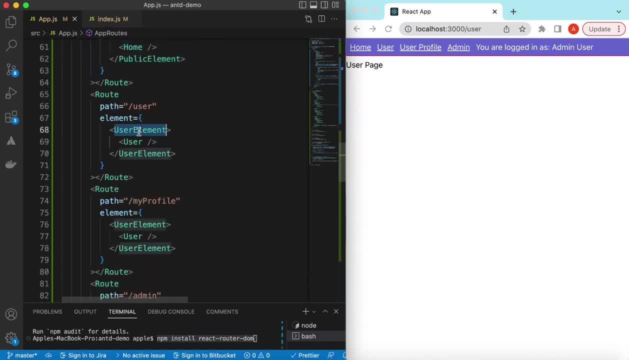 public, then this will be accessible for all users, and if it is of user element, then it will be accessible for the normal user as well as the admin users, and if it is an admin element, then it will be only accessible for the admin users. right, and then? here we have defined the different. 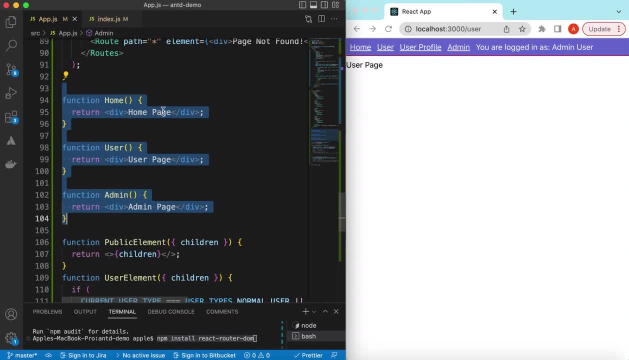 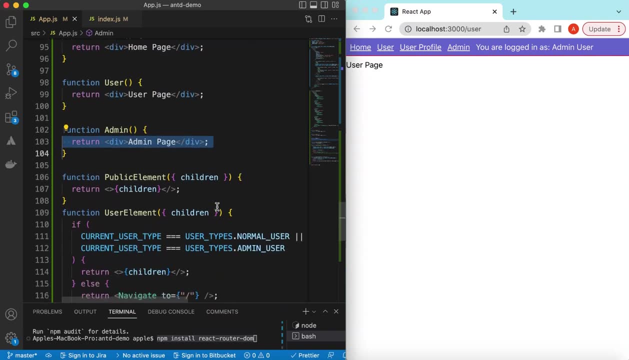 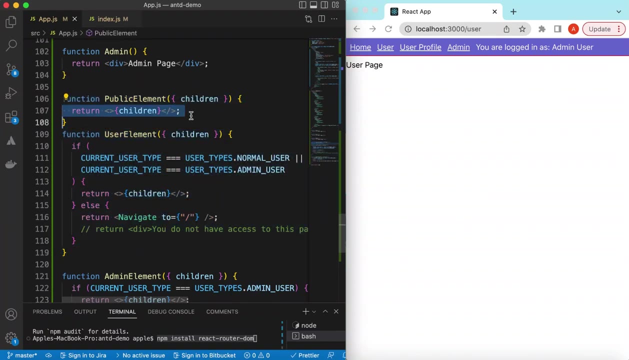 pages. so for now we just defined the only divs. but in actual applications you will be defining a whole page here, whole page here and whole page here, right, and then at the end we define these elements. if it is public, we are returning all of the children, whatever the page is inside that we 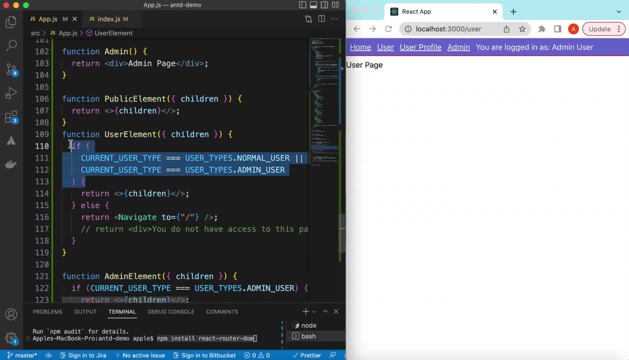 are turning that and if it is a user element, then we will first check if the user type is normal user or the admin user, then we will returning that particular page. otherwise we will be navigating to the home page and in case of the admin, uh, we are checking if the user.